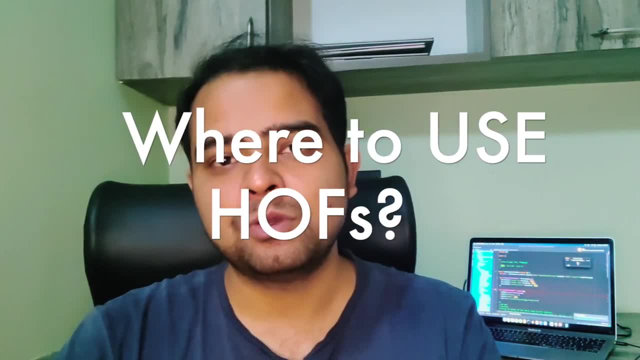 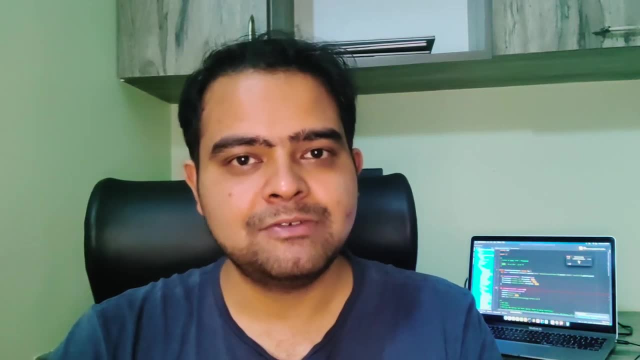 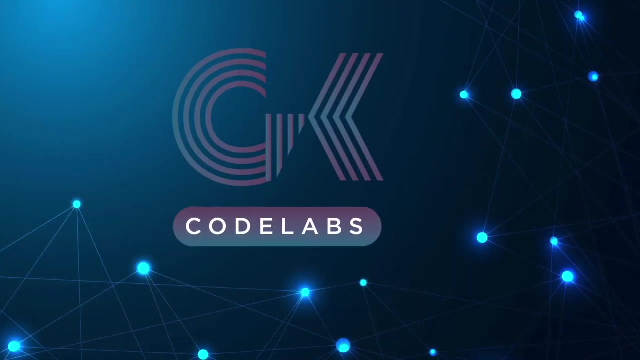 which, if comes to us, we should think of using a higher order function. so let's jump right towards the use case and see what do we have to achieve and where are we going to use higher order functions. so let's discuss a use case where just next step we have to do a higher order function. so let's discuss a higher order function. 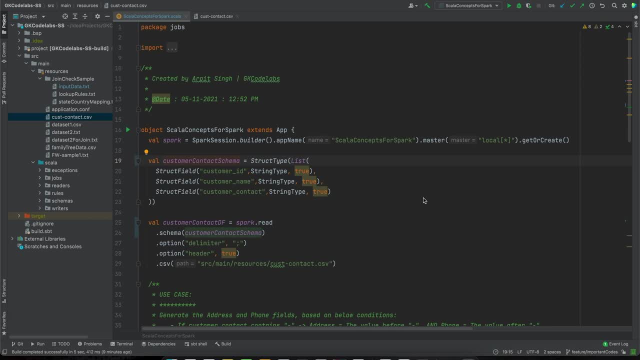 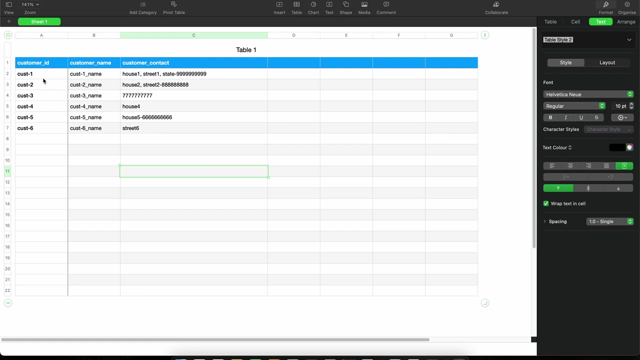 higher order function can be something for us to think of. let me walk you through the data set first. what data sort of? we have? small data set. just focus on the requirement. so just, we have three fields. i have kept to the minimal because you just have to focus on the requirement. 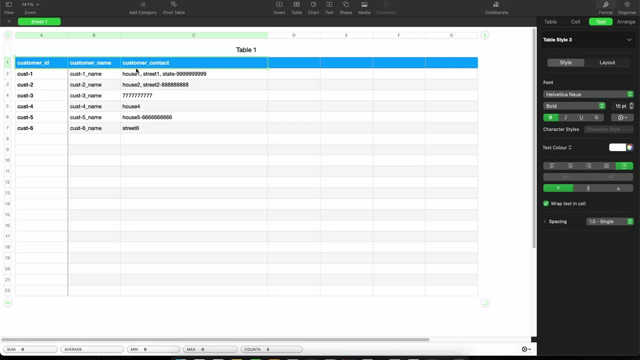 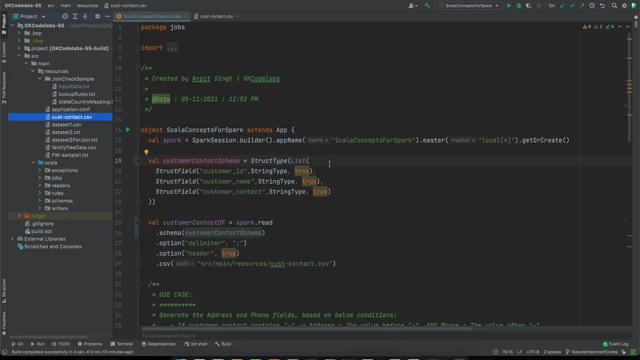 so we have three fields: customer id, customer name and customer contact. and we have six customers and their name and their customer contact. now let's see what's the requirement. i have kept them as a comment in the code itself. so, if you can see, basically it's nothing much. only i have initiated a spark session and this is the schema: id, name and contact. 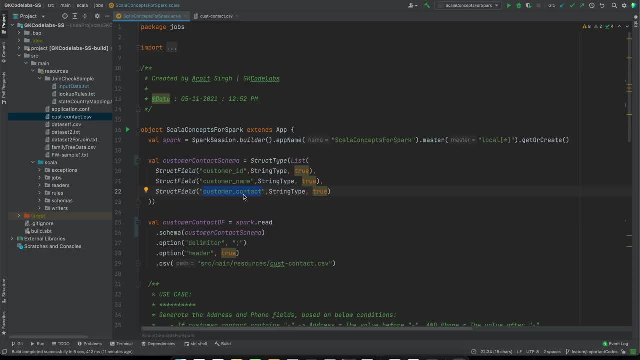 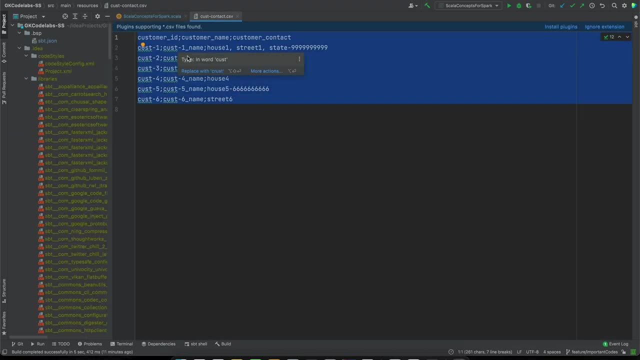 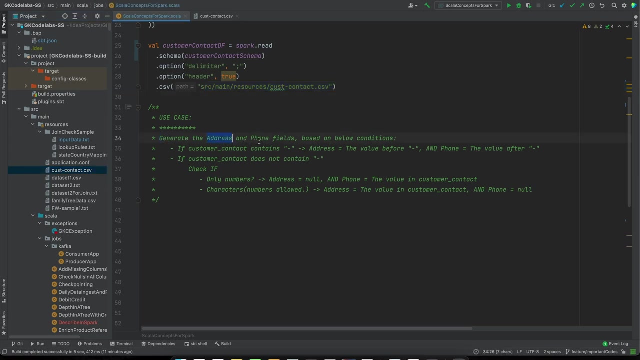 that we just sorted it out. so let's see what's the requirement. saw id, name and contact and we are reading this file. i have kept this as csv in the repository itself so you can see here how the use case says. we have to generate an address and the phone field. 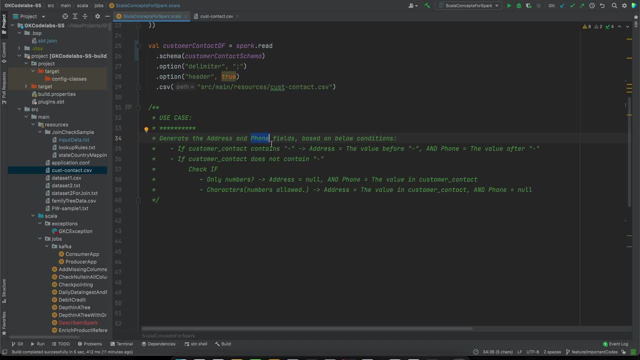 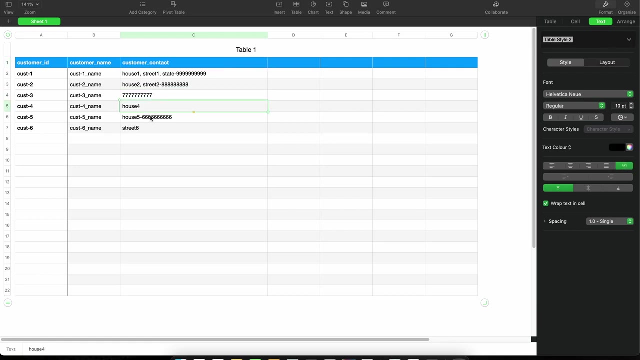 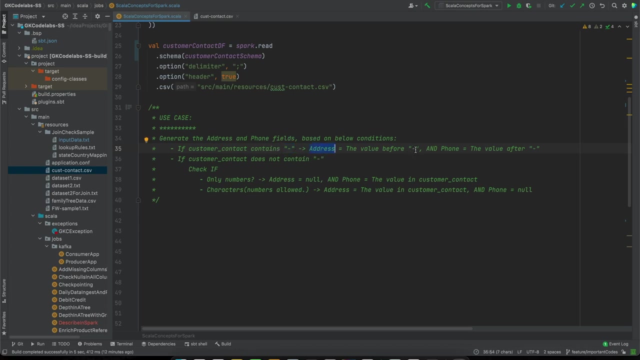 the address and the phone contact of the customer based upon the below condition: if customer underscore contact, that is this field. customer underscore contact if it contains a hyphen. right, you can see some places it has hyphen, some places it does not have an hyphen. so if it contains an hyphen, then address would be the value before hyphen and the. 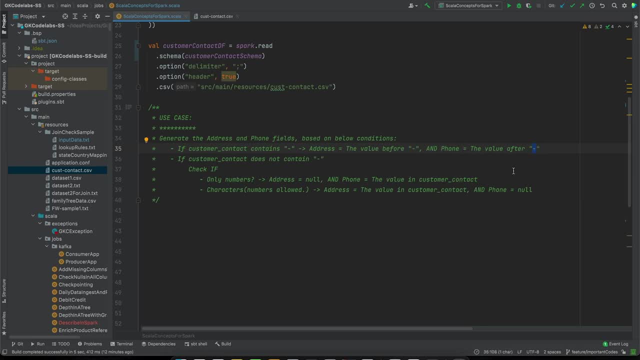 phone will be the value after hyphen. just to recall, we are trying to see the scenario where the higher order functions can be somewhat of use to us. so back to the requirement: the value of phone will be the value after hyphen. now if customer contact- that we just saw- does not contain a hyphen. so if it does, 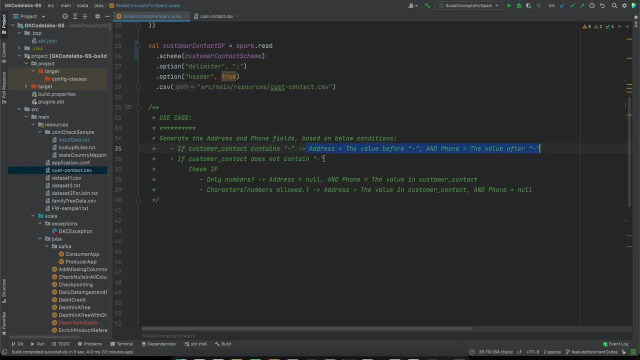 contain a hyphen. this we what we just discussed. if it does not, then we have to check again if it has only numbers. if it does have only numbers, then the address will be null, assuming that there is no address, it has only numbers- and the phone field will be the value in customer contact because it does not have any. 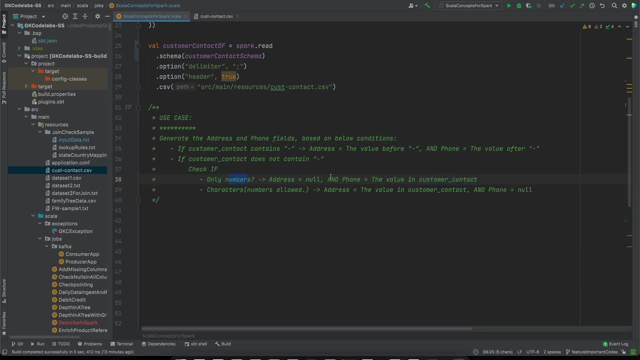 hyphen and all and it has only numbers. so assuming that it will be the phone number itself. otherwise, if it has characters, numbers are allowed anyways because in address there might be numbers. in that case the address field will be the customer contact. assuming that, because there is no hyphen first of all, and that is the reason. assuming that. 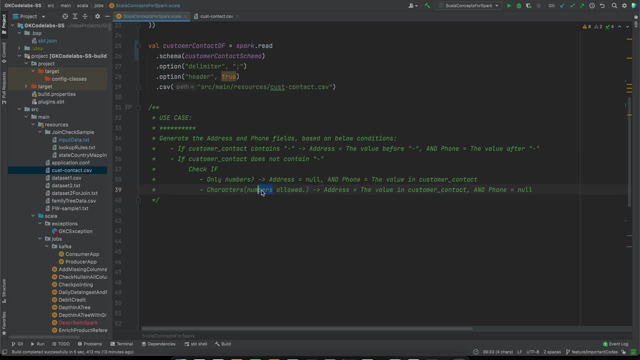 in case there are characters, numbers are allowed anyways, but everything will go inside the address and the phone will be null. so that is the basic requirement. if you have got it, fine, otherwise just rewind the video since when I started explaining the use case and then come back to this point. now for this. 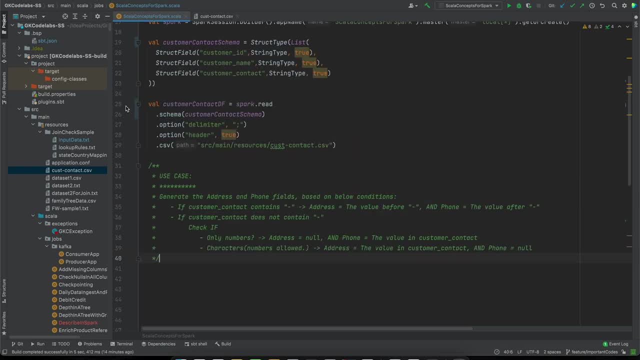 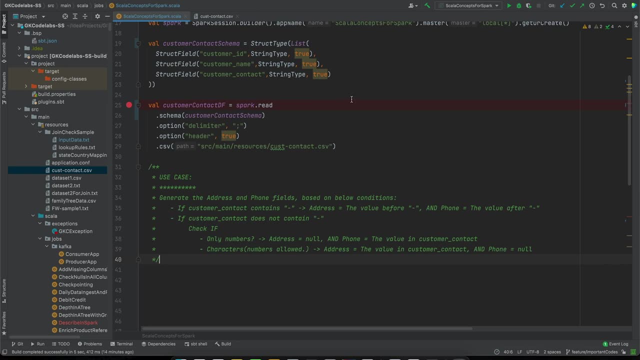 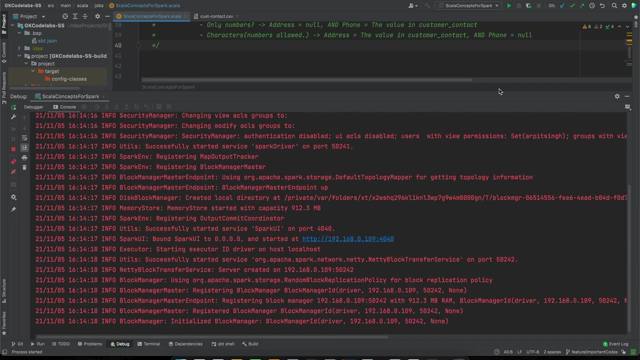 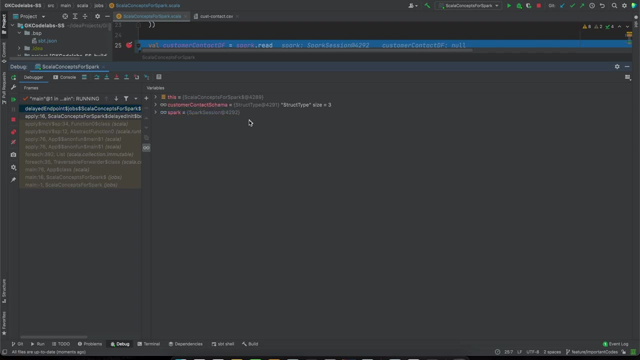 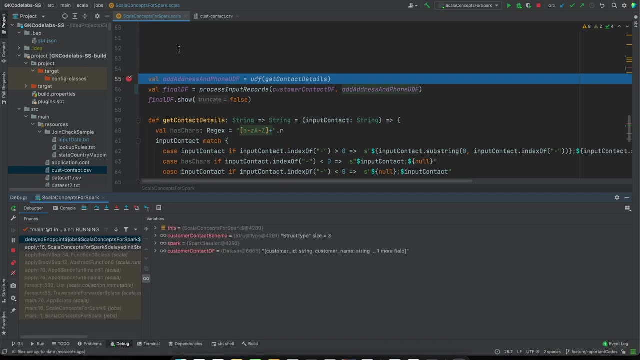 easily we could do. let's see what we are getting in this and put println somewhere and try to debug this println just for, like, if you don't have any successive code, but I do, so I have just put println in any next step segment, so let's move ahead so that this get calculated. and coming back to here, 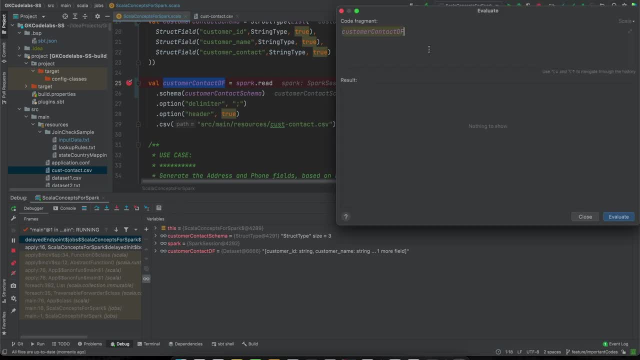 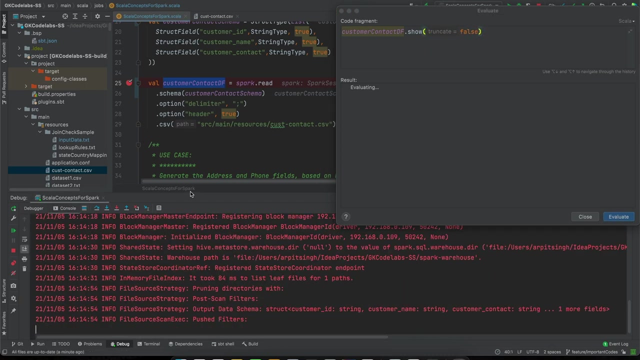 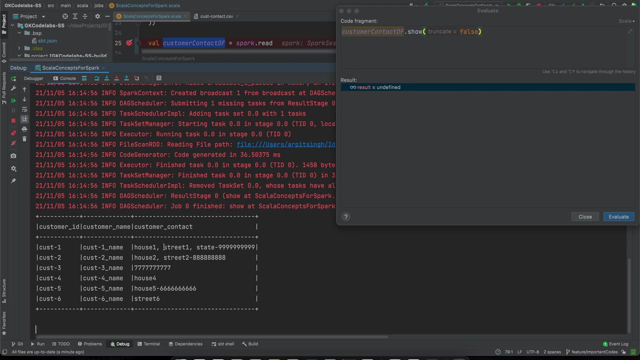 let's see what we are getting here. evaluate for this so you can see our file is getting read. main thing is customer contact. now, one way to do is because you can see there are multiple conditions, that is, their hyphen is there and not any hyphen on on top of that as well. is there only numbers, or are they numbers? 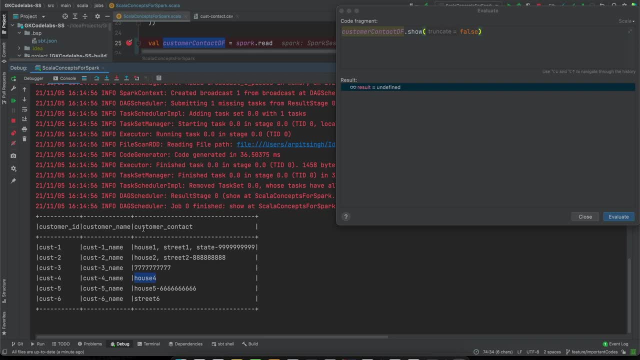 along with text. accordingly, we have to segregate this field into a number of ones, and this means that the present case that we are done here is not a hyphen. so we don't need to do anything with the previous one. so we don't need to do anything with the previous option. so if you 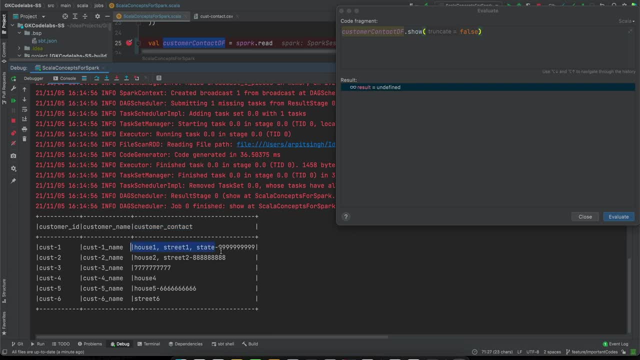 don't have any hyphens, as they are not visible. it is okay that you select them and then fix the addresses and the phone numbers right. so one way is to just directly go with with column splitting and something like that, but there are different condition. so in such cases the higher order functions are one way to think of. 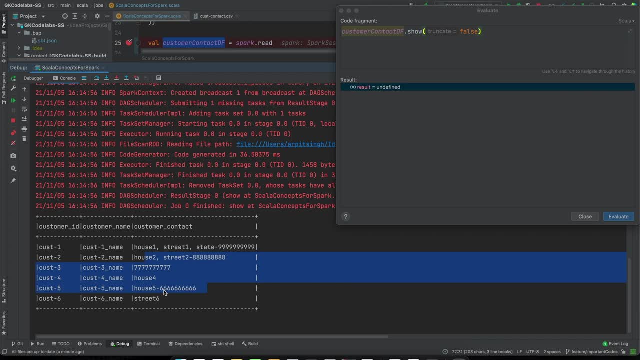 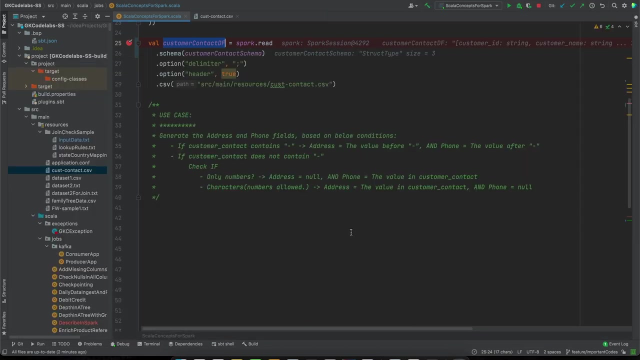 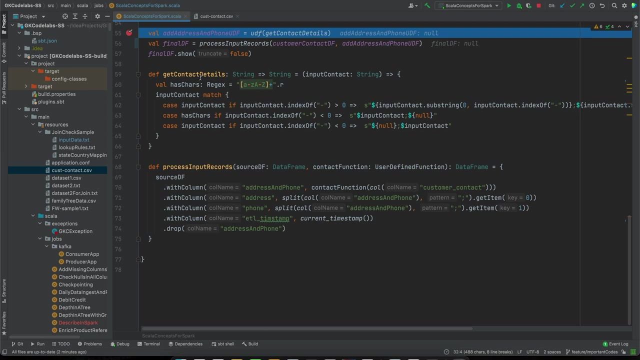 you can anyways work without them, but how they are used in a spark application. this is the exact scenario where you can think of using higher order functions. let's see how. so see for this requirement what I have done. first of all, I have created a get contact details function. before that, let us recall, I 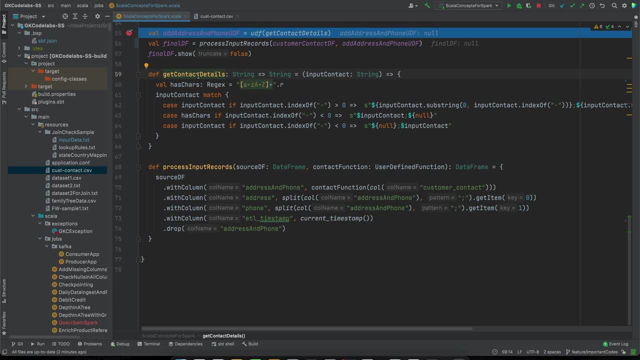 know you, every one of you, already are aware of higher order function. that's why you are here. a higher order function is nothing but which takes another function as an input, the master function, for that is a higher order function. so, coming back to the point, let's say there is a function, get. 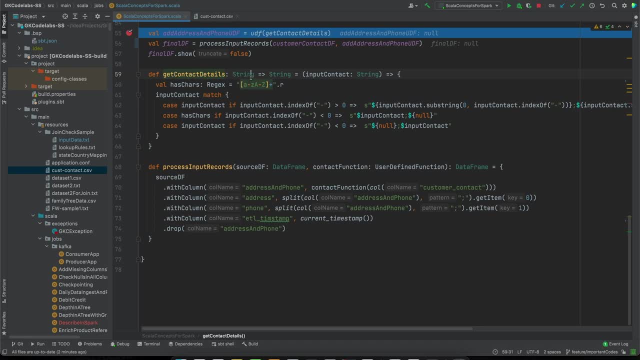 contact details that I have created, which takes a string and again returns a string. right, this is a function: takes a string and returns a string. now, given a string to this. we have a one regular expression as it. if it has characters, now see how we will use it. 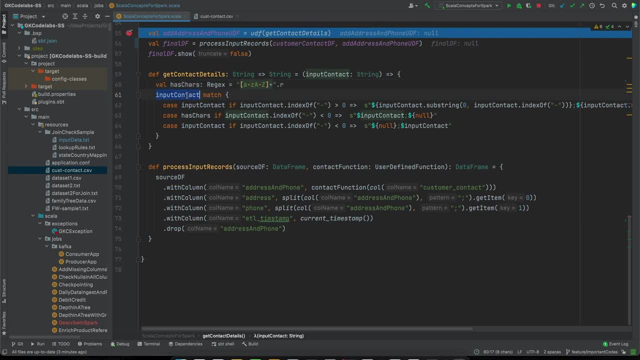 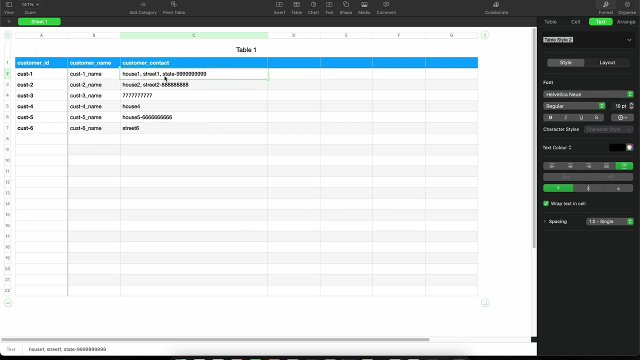 now for each value. if we have, for say, for customer contact, each value is one value in one row for this, that is, house one, street one and this, this complete value. what if we create a function that takes this value and evaluates what will be the- in this case, this part- and what will be the phone number- in this case, this part? 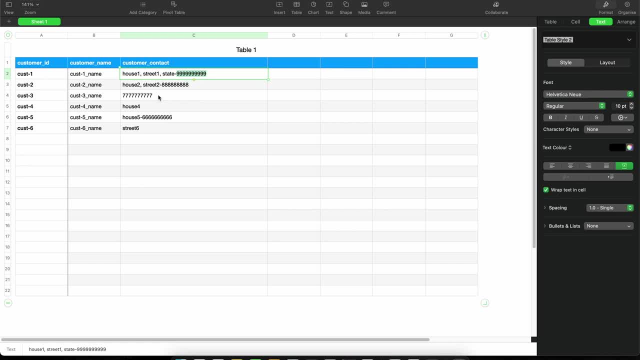 again, it takes each value, like for this and, based upon the requirement, it evaluates what will be the phone number and address. in this case, for each value it will compute different values depending upon the business condition because, as our business requirement says, if it does does not have any, if it has only integers, then this should be assigned as a phone number. 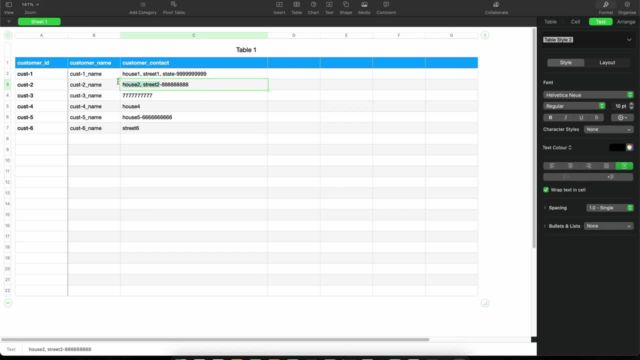 if it has hyphen, then this should be assigned as address and this should be assigned as phone number. if it does not have any number, then this should be assigned as address and phone number should be null. so, accordingly, what if we have such a function that we pass the values of 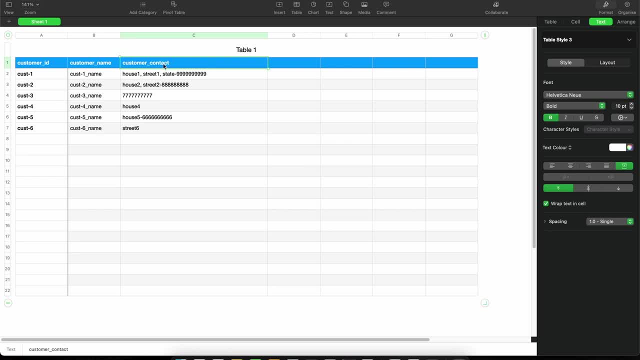 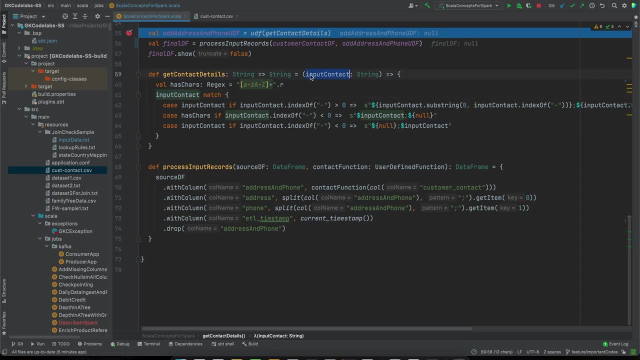 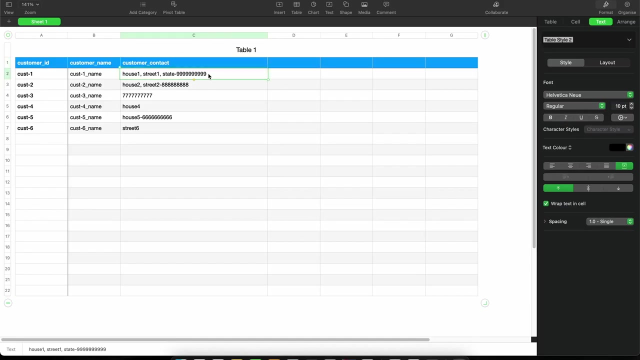 customer contact and that in itself calculates what will be the address and what will be the phone number and returns only the exact value of two columns: address and phone number. right, so, uh, somewhat similar. uh, i have done here. so this will be the input. contact will be why it is string, because this will be the value of each cell one by one. 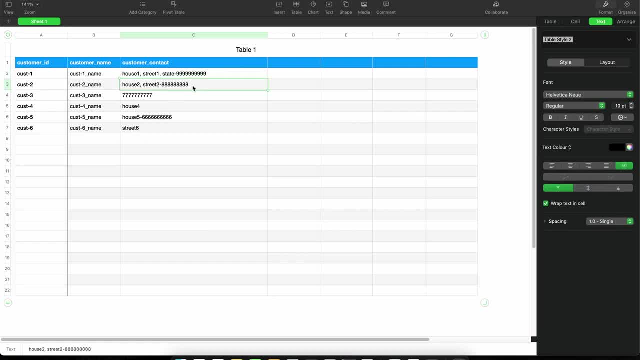 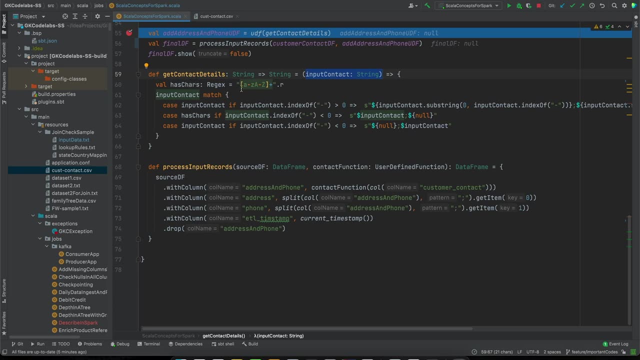 for uh customer contact. first it will go through this, then it will go through this. so this is complete string that we are referring to here. right? then we have a regex that only matches if it has characters. now see how we will use it- and then we are using a pattern matching on that. 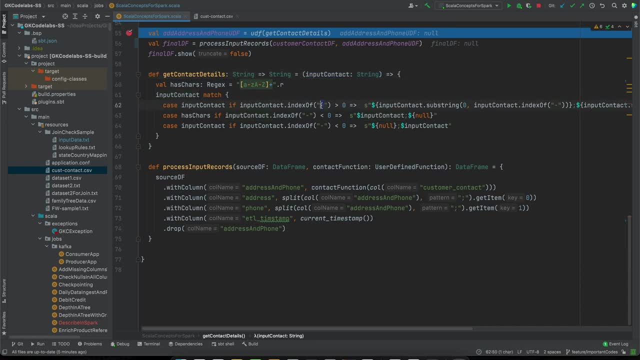 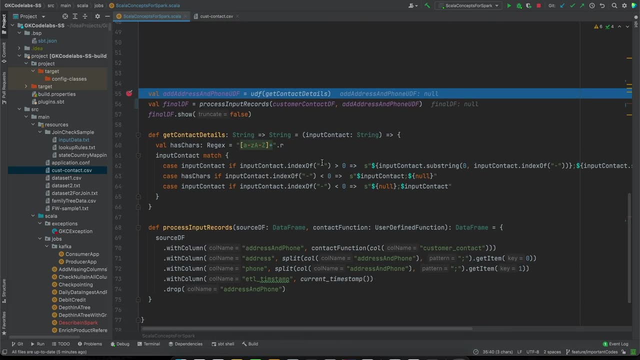 if it has any hyphen, as given in our use case. if it contains a hyphen, so that is what we are checking here. if it contains greater than zero, means index of this is greater than zero. that means if this, as a string, contains anything regarding this, then the index will be greater than zero. it will give you the index of. 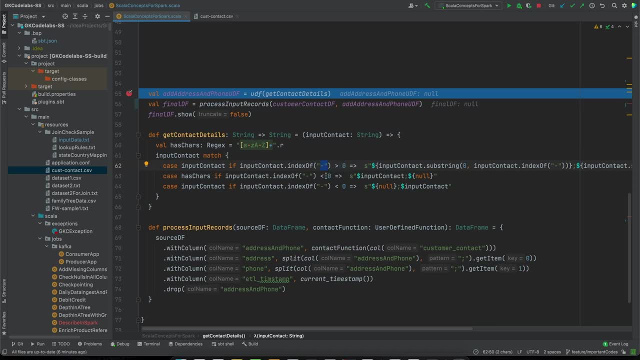 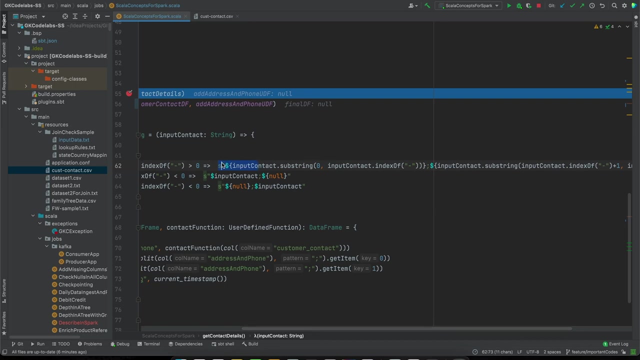 that if it does not, there will be no index and the value will be negative. that we will be checking in. next condition. so if it has, then what will be our return? we are sort of concatenating the address and phone number. later we will be splitting it. so our first value, which will be: 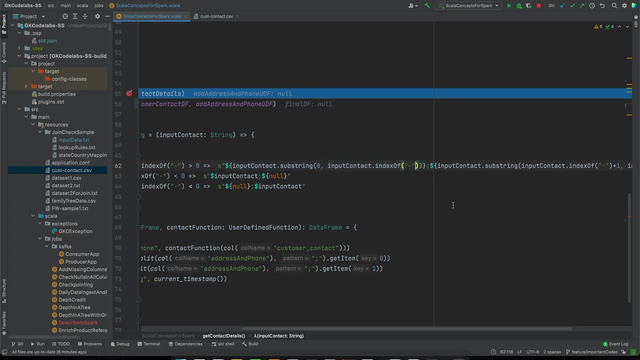 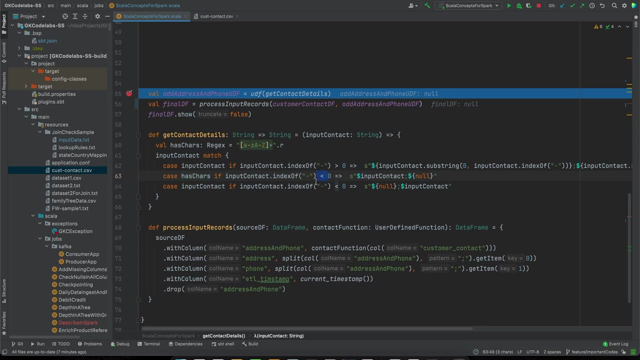 address will be from zero till hyphen and the contact will be from hyphen plus one till uh, the end, that is length. if it has characters and there is no hyphen, less than zero means there is no hyphen. and if only it has characters, not only. 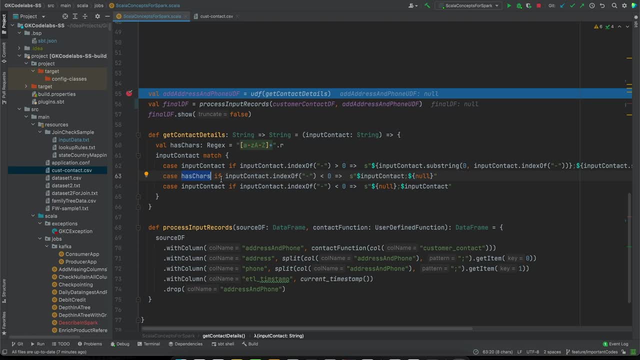 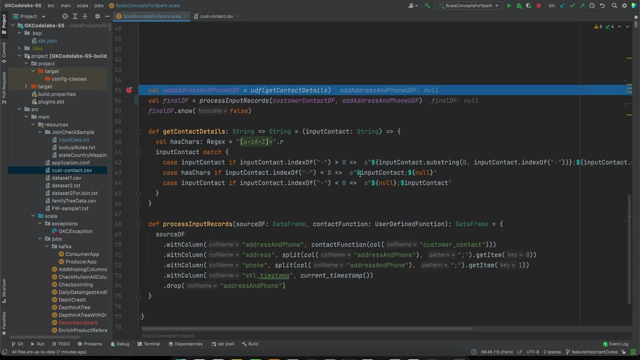 but uh, characters plus numbers, because here it is written numbers are allowed. your address can have numbers. so in that case complete thing will go into address and nothing will go into phone number. and if again it does not have any hyphen and it does not have characters as 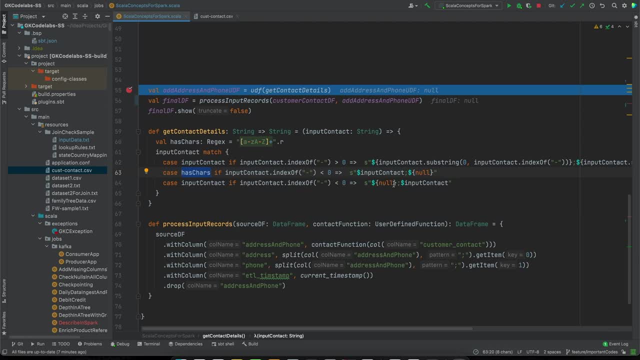 well then, obviously that is a phone number, so our address will be null in that case and the phone number will be whatever we are getting now this simple function we have created which takes a string, but our data frame does not give a string straight away. right? so what we have done? let me stop the debugger. 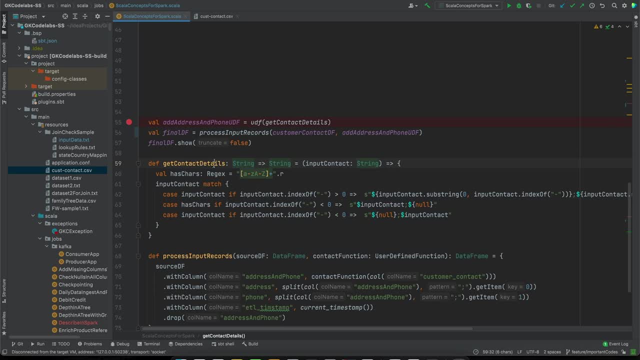 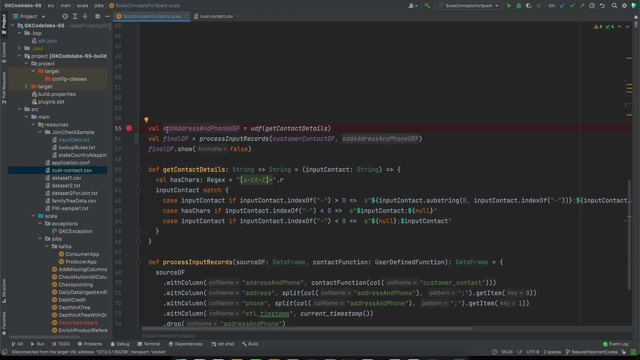 what we have done. from this contact details, we have created a udf right. this will be registered as a udf and the name of for that will be add, address and phone, udf. and that is what we will be using, uh in populating our final data frame. 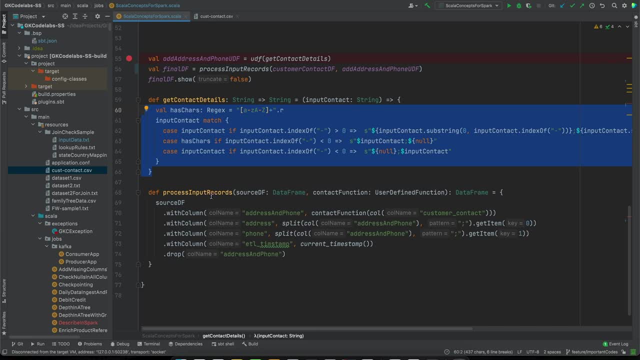 so how to use this. we have created another method. now coming to the point for this video where we are using the higher order function. now you can focus on this process: input records. this is a higher order function because it takes the input data frame and again, it takes a contact. 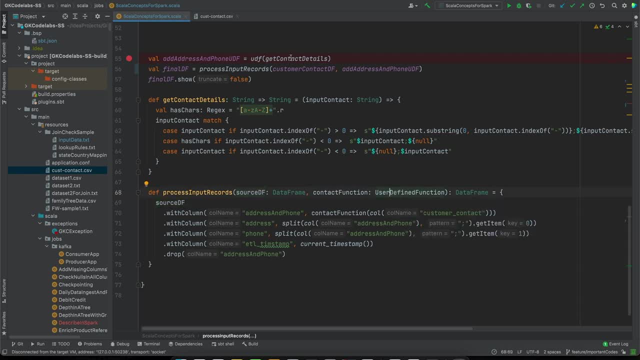 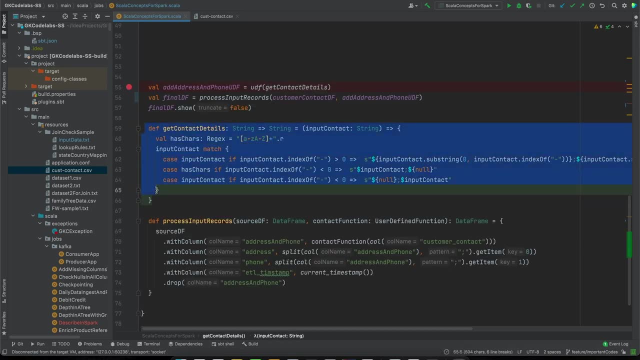 function, a user defined function. what is a user defined function? that is the contact details. now you can see this is again a function. so our process- input records- is taking a function as an input. so i hope things are making sense now. this function is using another function as an input and 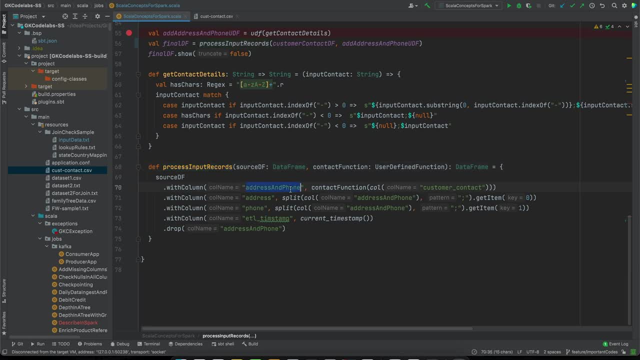 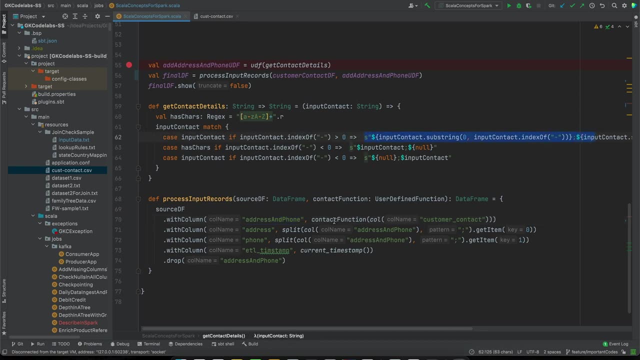 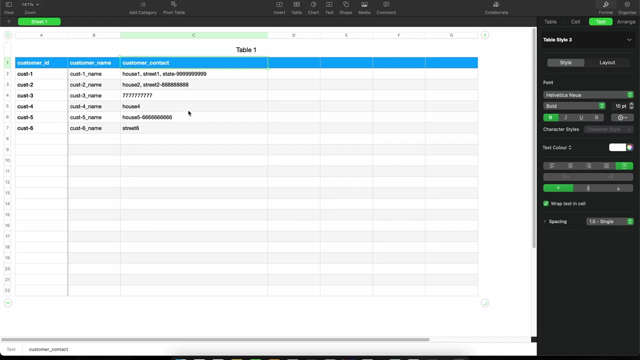 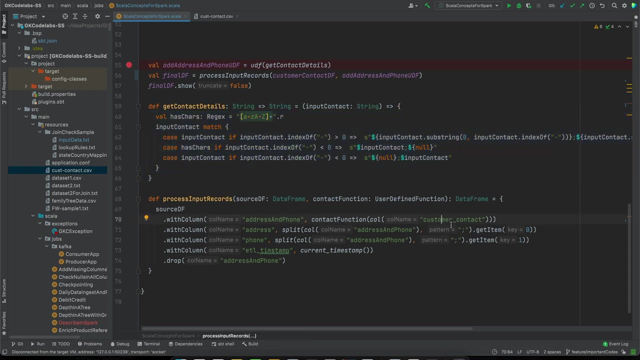 how we are using it. we are using with column because we know this will give a concatenation of address and phone. so we are just using this and passing the customer contact field- customer contact- and on top of that, whatever it has to do will be done in this function. we don't have to clutter our with column statements now, simply. 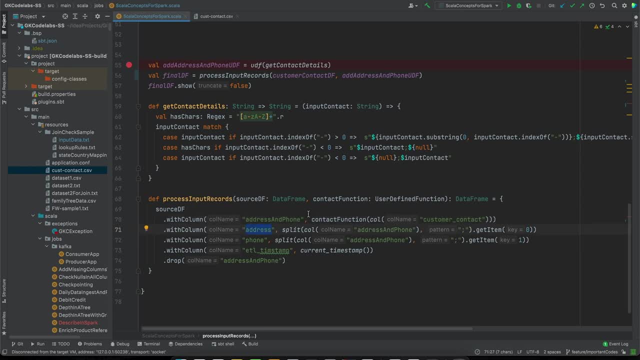 what will be our address? address will be the output of same field, but the first value. what is the first value? first value is, according to the given condition, whatever is coming first, separated by semicolon. okay, so separated by semicolon, get key of 0 is our address and get key of 1 is our phone and another. 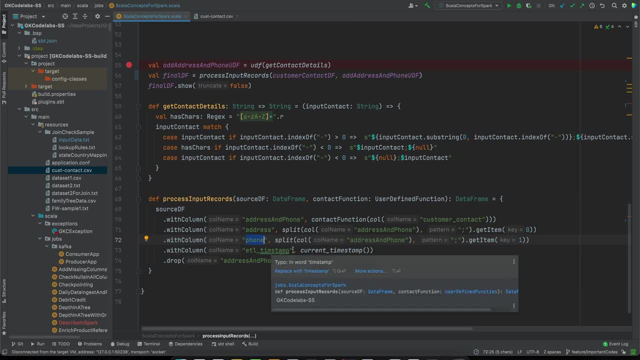 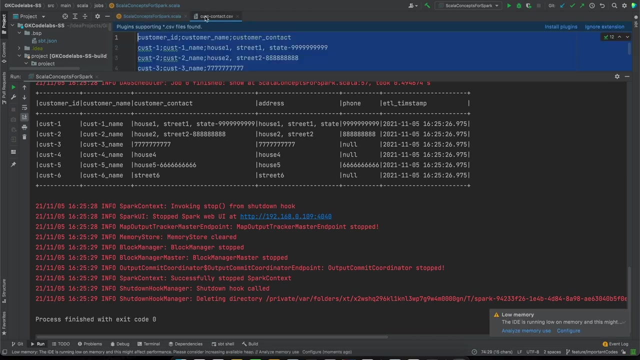 requirement, whatever requirement you want. i have added here like what will be the timestamp so we can add when this record got processed and we have already splitted and got our interested field. so this, which has complete information separated by semicolon, is not of use now, so i'm dropping it. okay, so let me run it and show you the output. so there you can see. the input was this. 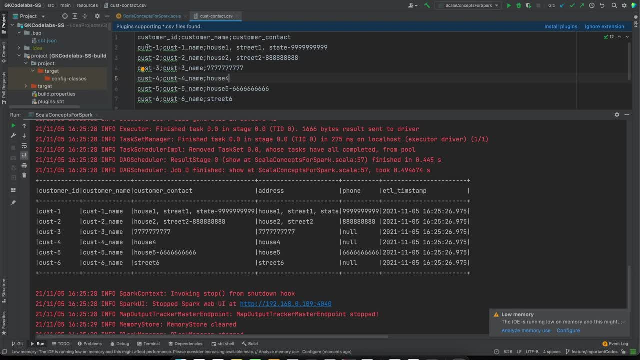 okay, so here when it has hyphen, it gives whatever is before as an address and whatever is there after that as a phone number. and similar thing here, street two and phone number. and if there is nothing and there is no alphabet as well, this is coming as an address. but i think this should. come as a phone. so that's one of the points here, following a line in case we do not provide address and computers can put anything we say to one another. but one other thing: if there is nothing, then this is miles less available. so number two: if a message has voice-to-be distress bar or if something has info income, and i could also not have info. i could often do it, but i am happily comfortable that i be using on cabeup as one in my lab. i could probably all white time. thanks for watching this video. that is full-time. my name is muamad alupabalab, mother of two years, but i have questions. that is some from last month, but if you have questions, 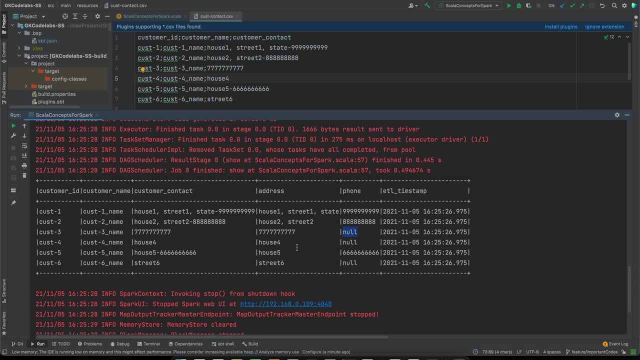 phone. uh, so we'll fix this. rejects. but apart from that, if there is nothing as a, if there is a, an address only, so our address will be populated and phone will be null. and in such cases, where there is a hyphen, there will be the address and phone number will be separated. and again, if there 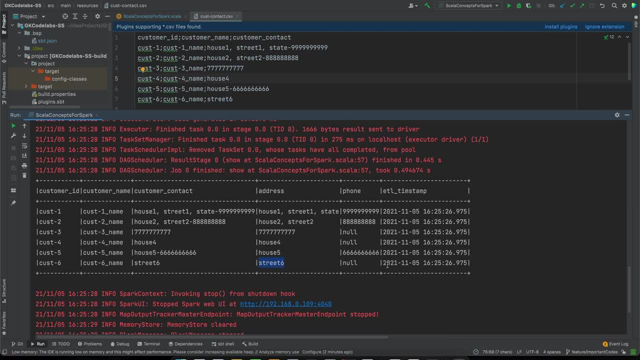 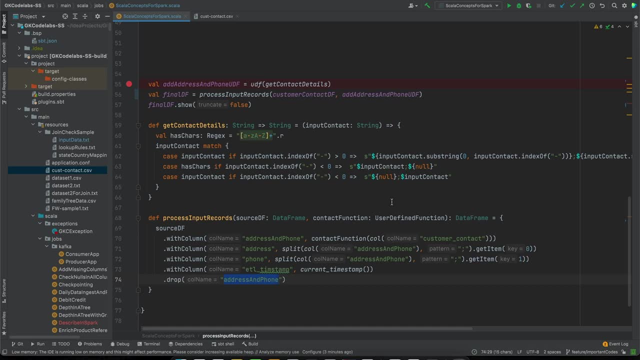 is no phone number, the phone number will be null and that is how it will be separated in. so the main thing to note here is where you need to populate a column based upon different conditions. it's not just like you have to concatenate some column for every field you have to check within. 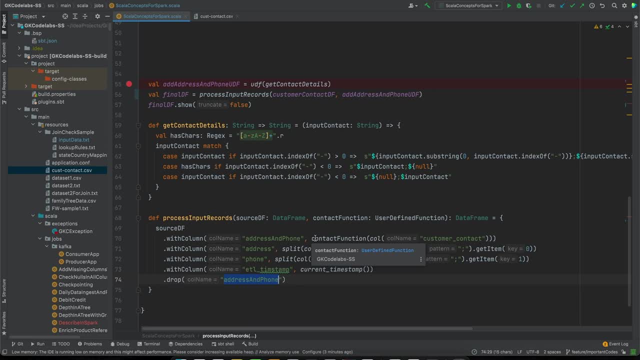 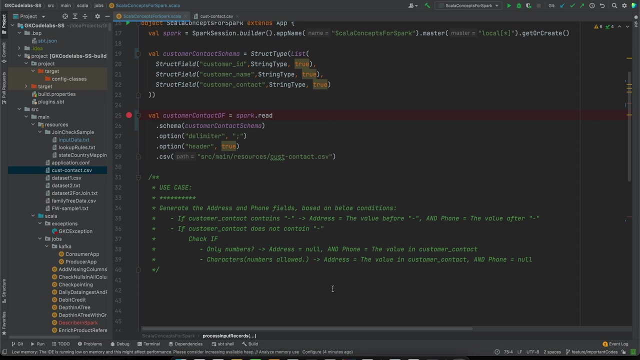 that in that case, the higher order functions are a way to think, the approach of. so we'll be bringing up the use cases for more scala concepts like currying, partial functions, partially applied functions, more similar scala concepts which, as you know, spark is based upon scala, and these are the questions very importantly asked in big data. 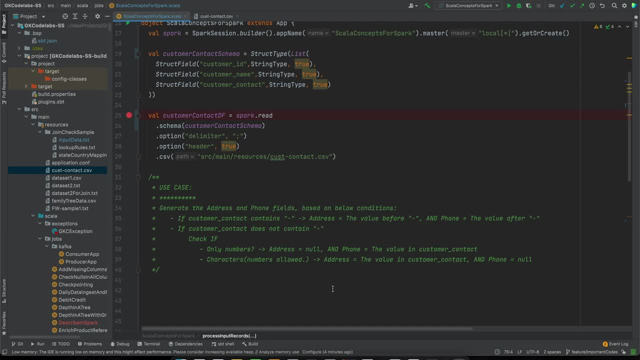 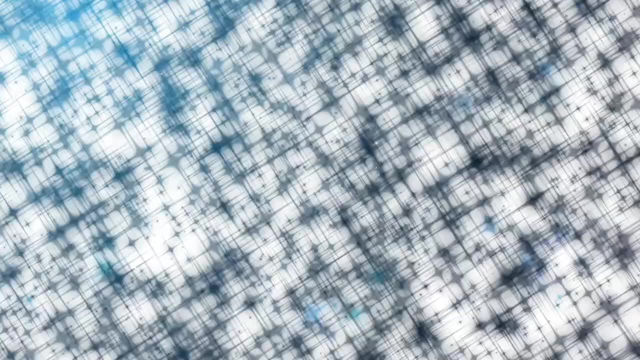 interviews that. where have you used this concept? please hit that like button if you really liked the video, and please subscribe to gk codelabs if you have not already done. thank you guys, see you later you. 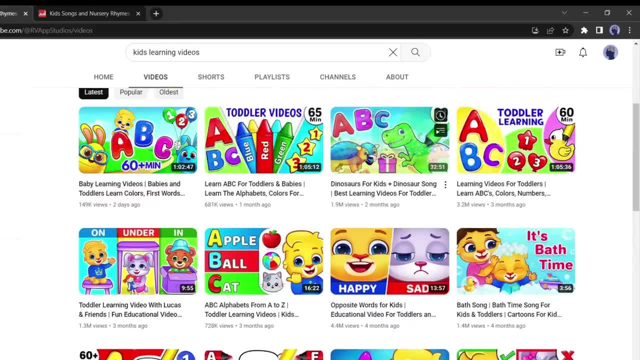 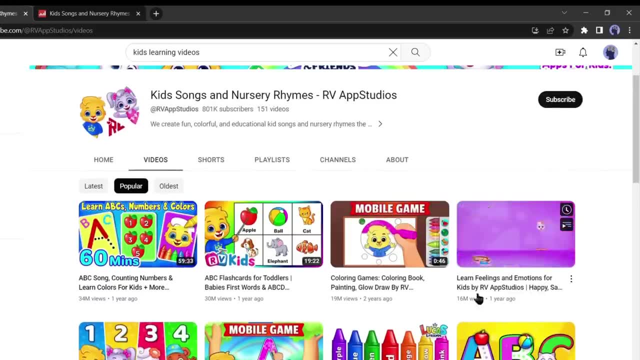 This YouTube channel is making a huge amount of money by creating simple kids learning videos. They use 2D animations and some of their popular videos have received over 30 million views. If we check their channel on Social Blade, they have more than 800k subscribers.